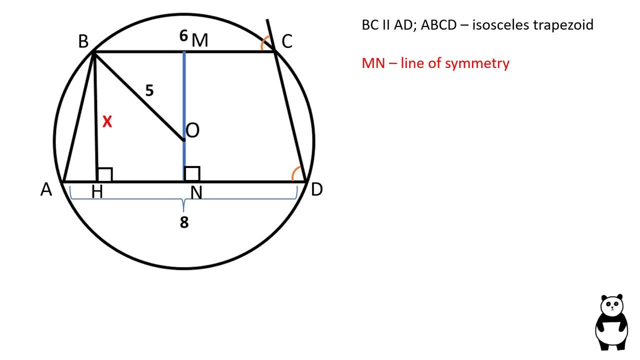 the line of symmetry goes through the midpoints of the bases and is perpendicular to the bases of the trapezoid. The line of symmetry will also go through the center of the circle Triangle. BMO is a right triangle. OB is equal to 5.. BM is equal to 3, since M is the midpoint of BC. 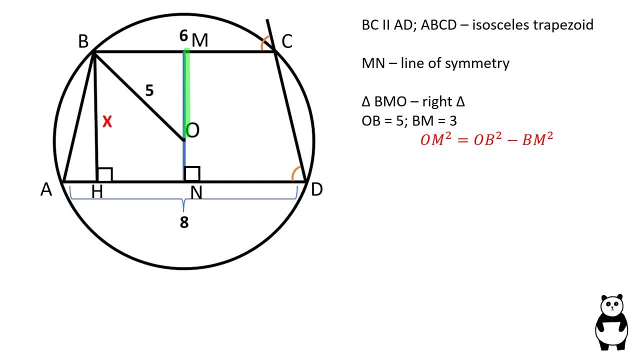 We can find OM using the Pythagorean theorem: OM is square root of 25 minus 9, which is 4.. Let's connect point O to point A Triangle. AON is a right triangle. OA is equal to 5.. AN is equal to 4, since N is the midpoint of AD. 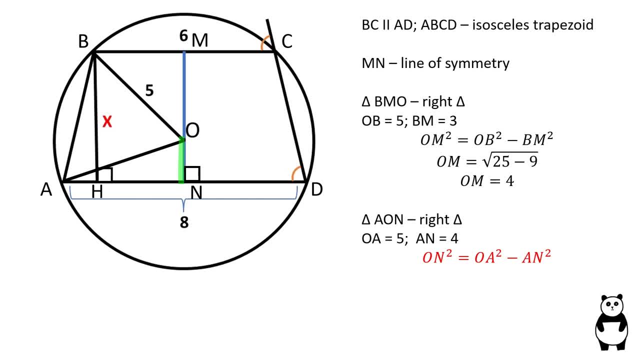 We can find ON using the Pythagorean theorem: ON is equal to square root root of 25 minus 16, which is 3.. mn is equal to om plus on, which is 7.. And since mn is equal to bh, x is also equal to 7.. If you found this video helpful, please consider. 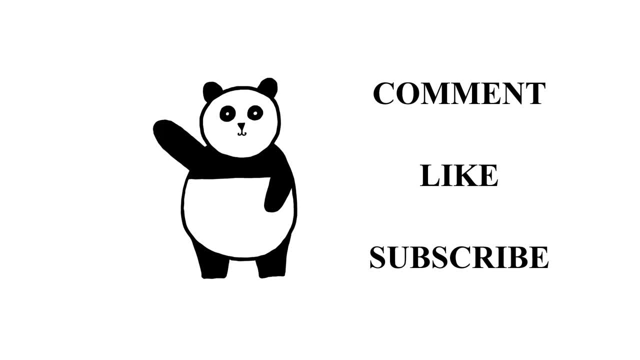 to subscribe to help my channel grow. Thank you. 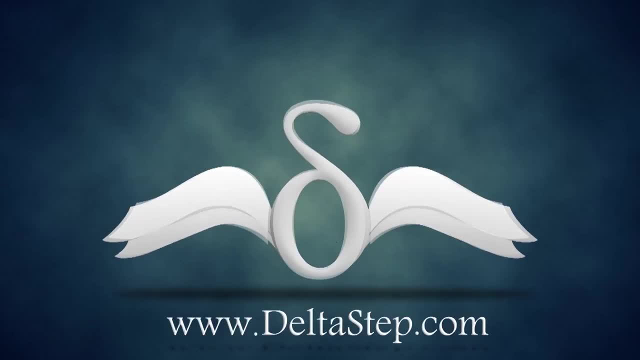 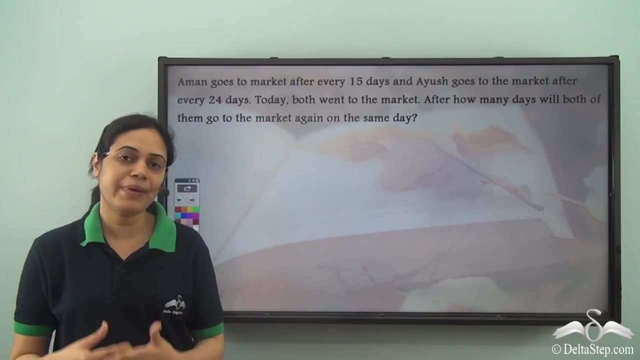 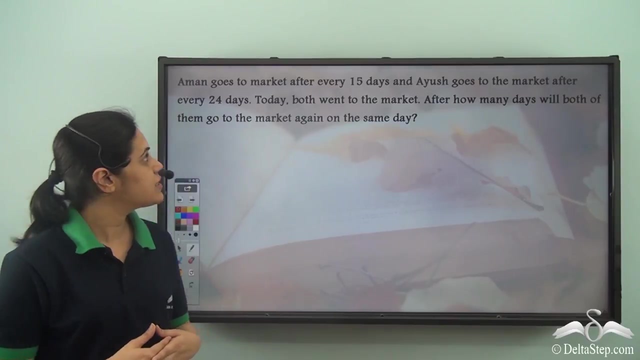 We know that mathematics helps us to solve many problems, So we have this word problem here. Let us see how we can solve it using mathematics. It says Aman goes to the market after every 15 days and Ayush goes to the market after every 24 days. Today both went to the market. 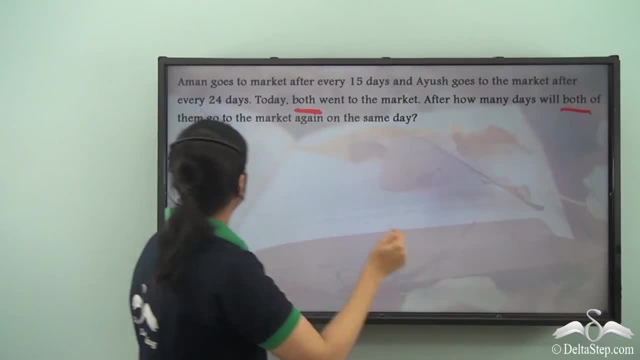 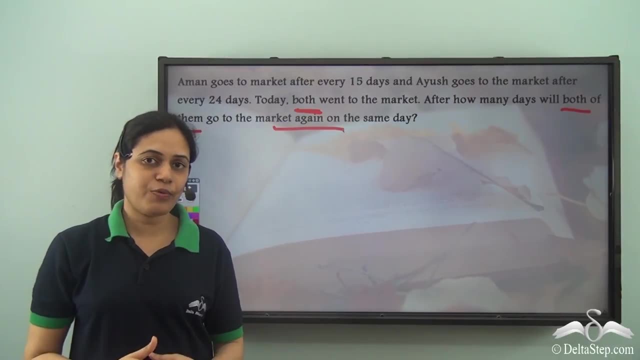 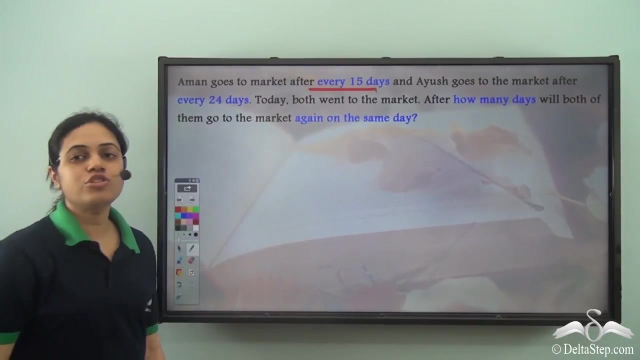 After how many days will both of them go to the market again on the same day? So whenever we have word problems we need to look at certain key words or important words which tell us what do we need to do with the word problem. So over here we have that Aman goes to the market after every 15 days and Ayush goes after.